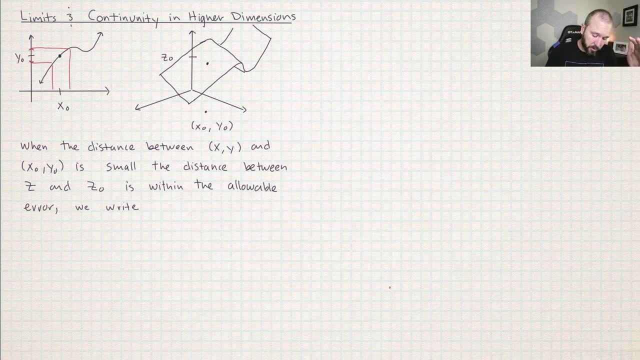 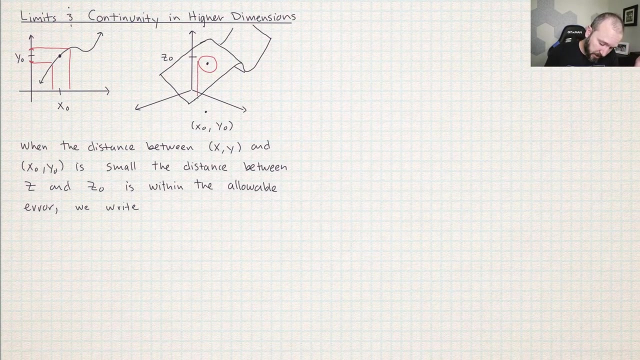 Now in Calc 3 I'm going to use x's and y's to produce z's. so this means I need to require that all of the z values stay within some allowable tolerance around z naught and then trace that back And this will give you. 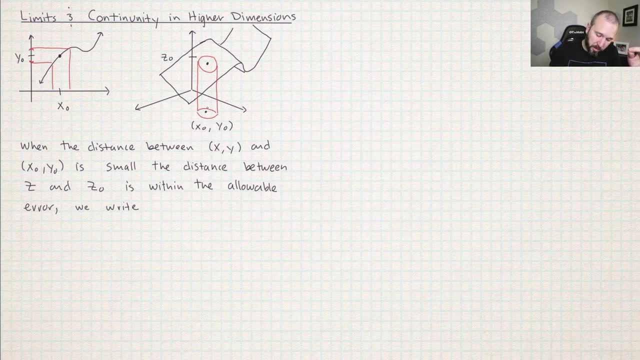 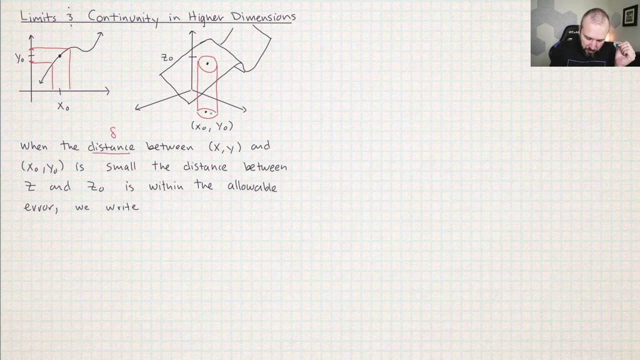 a range of input values that will always keep you within the allowable tolerance of z, Requiring that your inputs be within some small distance. we call this small distance delta. In the picture, delta is the radius of this circle or the radius of this interval. that would be delta right there. 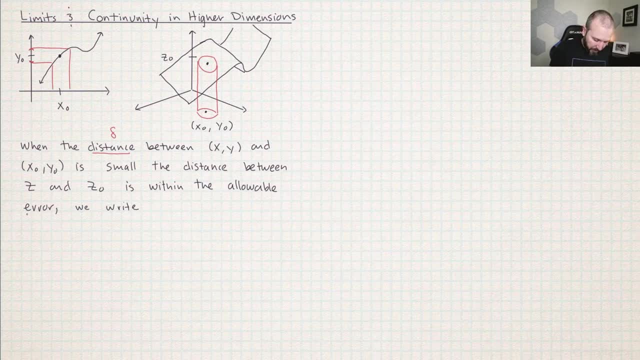 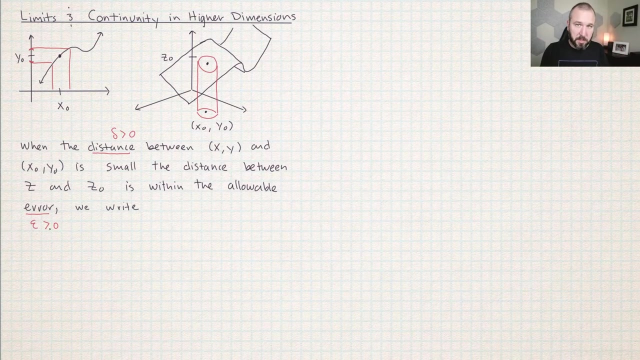 And then the allowable error. we're going to call that epsilon. You'll see, usually when people write these they'll always put greater than zero symbols next to them. That's just to kind of remind everybody that these things are positive quantities because they always represent distance. 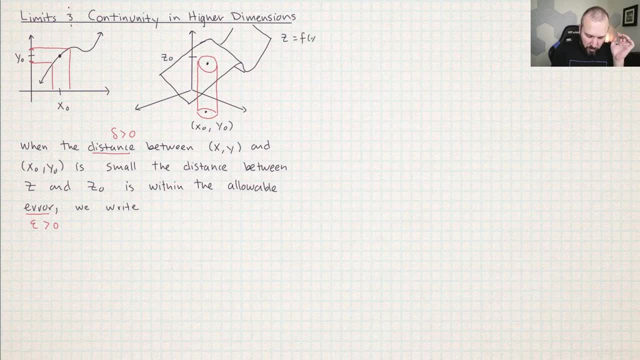 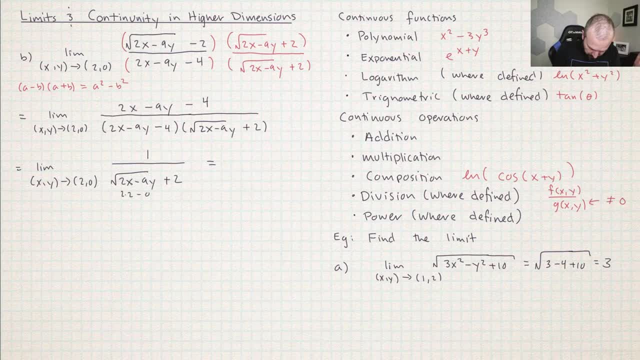 in. So what is this going to be? 2 times 2 minus 0.. So that's the square root of 4 right here plus 2.. So on the inside there, so in the entire denominator there, I'm just getting a 4.. So 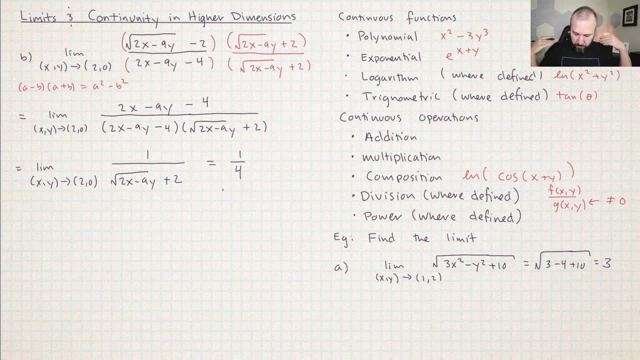 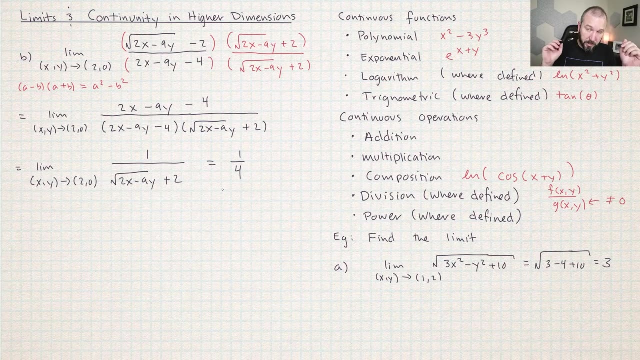 this whole value is 1, fourth. So you know this can kind of be a little bit misleading, as though limits always exist. It's actually that's not true. There's a whole category of functions for which limits at points are undefined, And I want to show you our main check when we're trying to 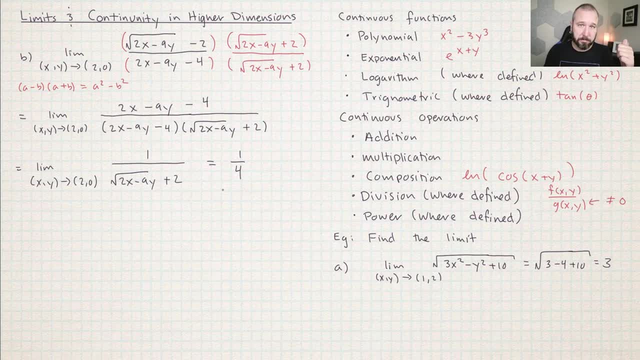 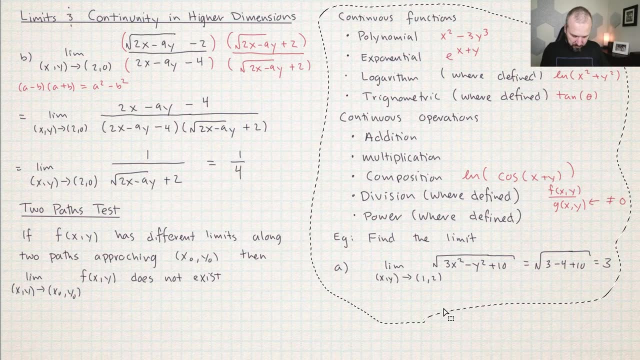 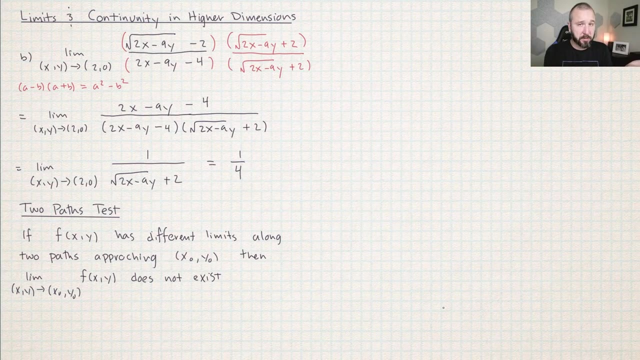 show that a function does not have a limit. We call this the two-path test for existence. So the idea is that if you calculate the limit along two different paths and you get different answers, then that means that the limit does not exist. You actually had this in calc 1 as well. It was just before. our domain was just the x-axis, So 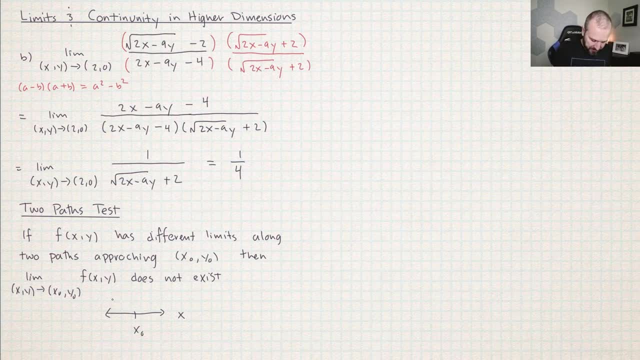 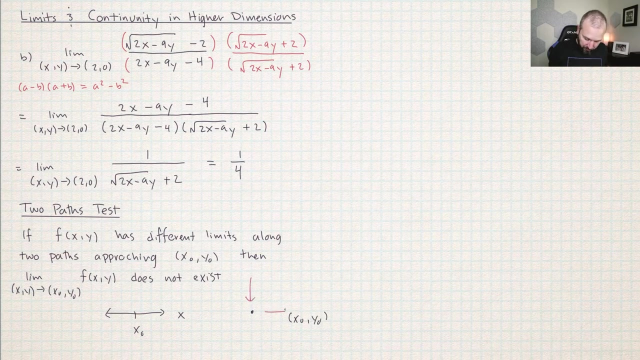 the only way that you could approach a point on the x-axis is either from the right side or the left side, So there's only two choices for the two different paths. But now that the domain is the xy plane and we're trying to approach a point x, not y, not, you know, there's lots of different ways. 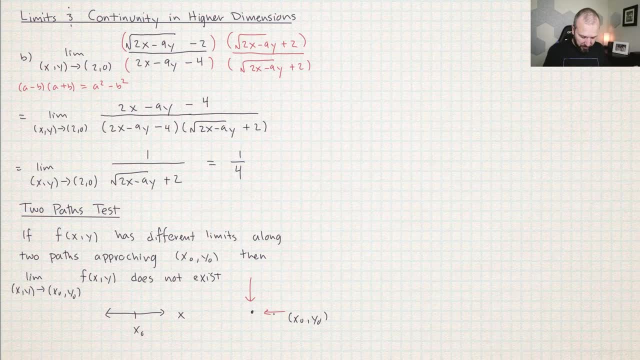 that we could approach that point, Not just these, like two, like right-hand limits on left-hand limits. Now you're allowed to approach a point on the x-axis. So you could approach a point on the right-hand limits, on the left-hand limits. Now you're allowed to approach a point on the. 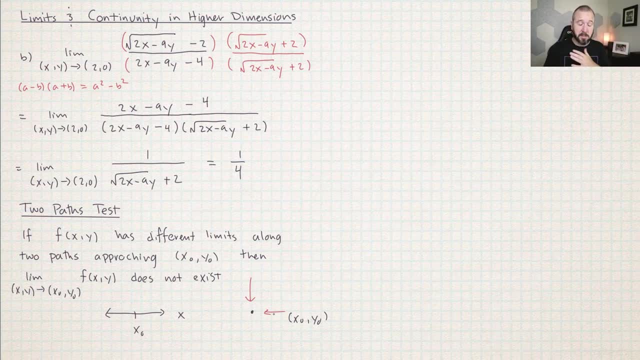 x-axis. So you could approach a point on the x-axis. So you could approach a point on the x-axis. So you could approach a point on the x-axis. Now you're allowed to come from any direction. If you get different answers, then the limit doesn't exist. 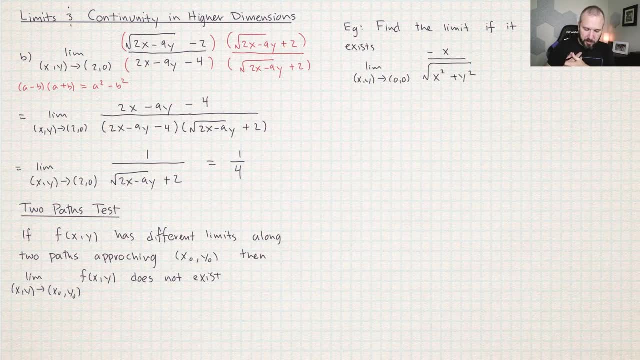 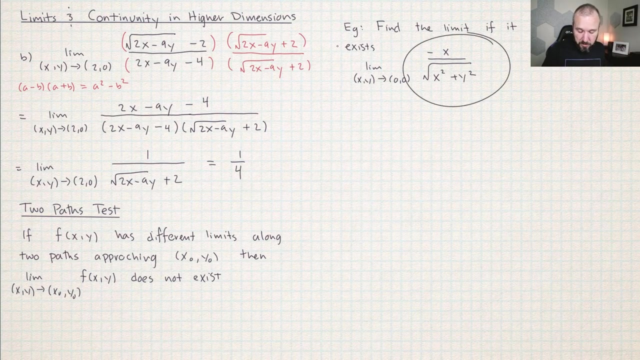 Okay, This is the classic example of the two-paths test And this demonstrates really why it's kind of easier for functions in higher dimensions to have limits that don't exist. So just have a look here at this function: negative x over the square root of x squared plus y squared. 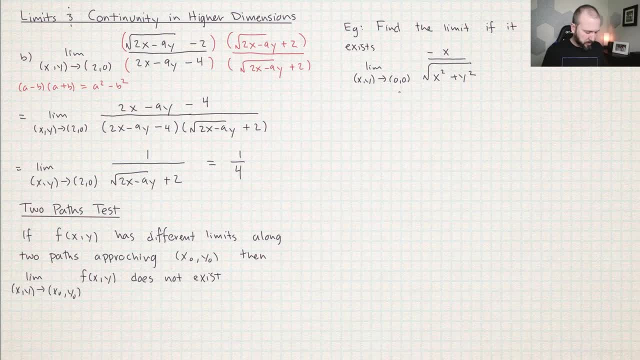 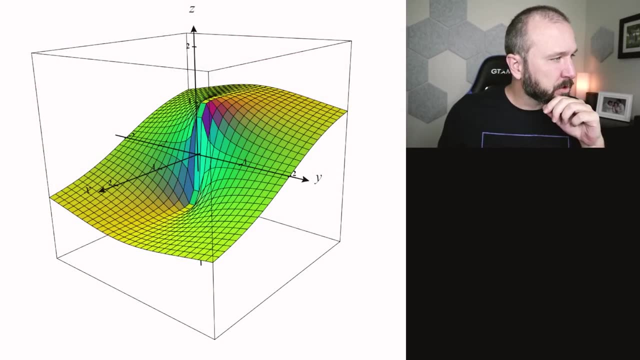 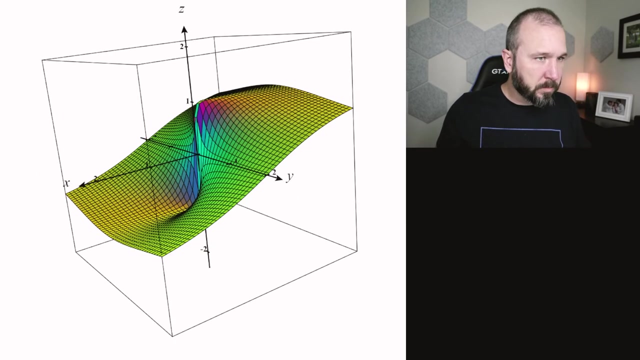 And we're examining by height of this surface around the origin. So I've got CalcPlot3D to graph it for us. So here's what the surface looks like. Let me just This is okay. So this is what the surface looks like. Let me just up the resolution here. Okay, That looks a little bit better, All. 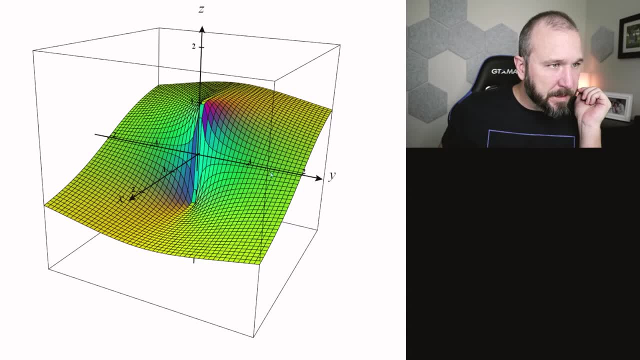 right. So if I'm going down the Y axis on either side, if I'm going down the Y axis, this surface, if I'm only on the Y axis, this surface, all looks the same right. It's going right towards zero. 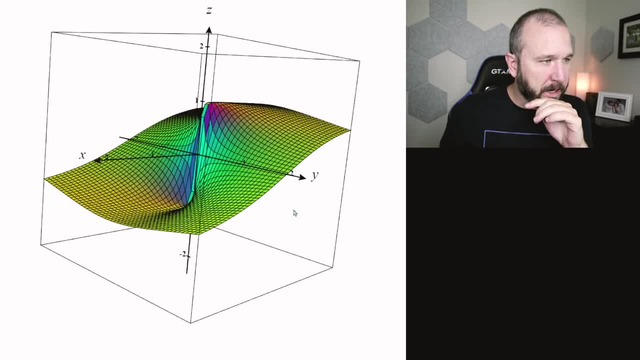 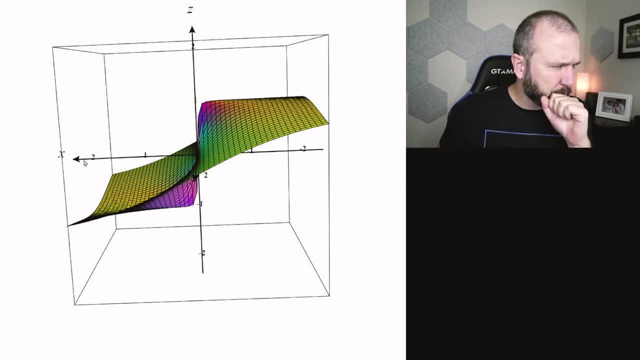 zero. Okay, All along that Y axis. But now if I look down the X axis, this is where the behavior is kind of weird. You can see, on the left side of this axis I'm getting closer and closer to negative one, And on the right side of this axis I'm getting closer and closer to positive one. So 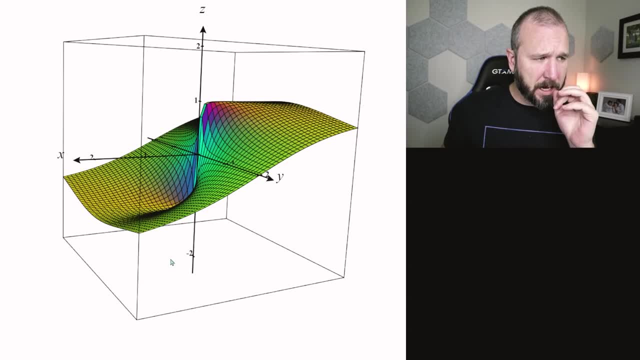 this is like really bad. I mean, this limit doesn't exist. First of all, along the Y axis. if you're going from the positive Y direction towards the origin, you're going to get zero. And then, if you're going, This should be the negative X side. If 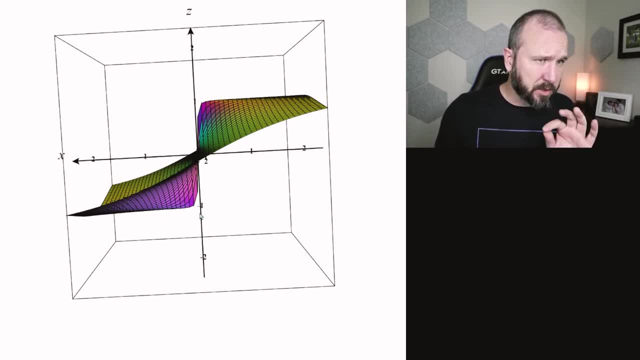 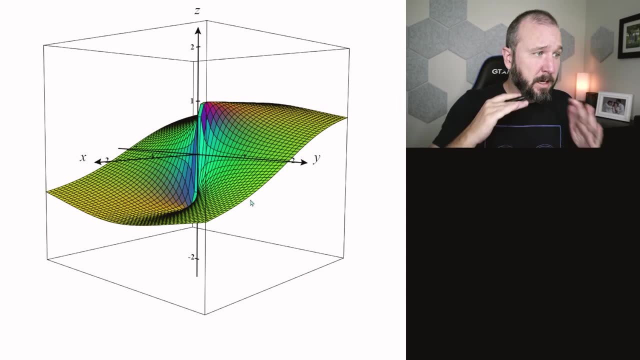 you're going down the negative X side, you should get positive one. If you're going down the positive X side, you should get negative one. So as I approach the origin, going along different paths in the XY plane, I get different values for that limit. So let me just show you how we usually 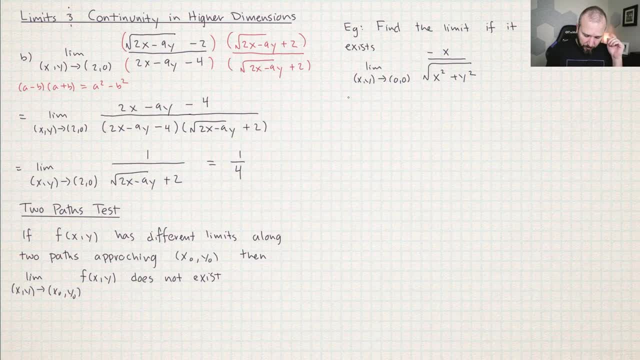 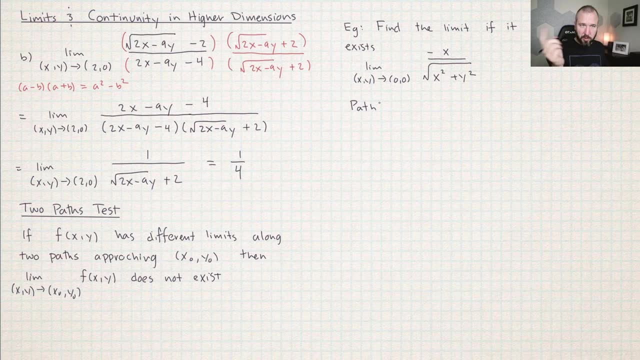 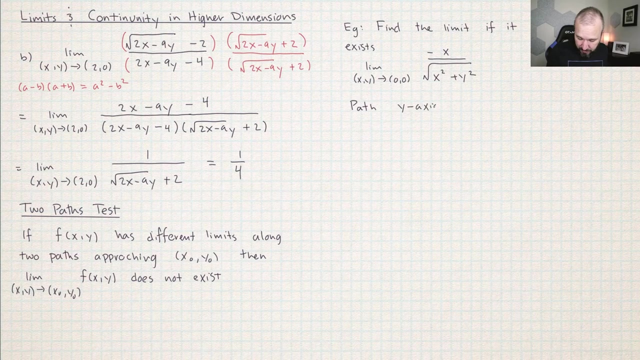 write that to solve this problem. Okay, I'm going to choose two paths. The first path that I will choose is, let's do that one along the Y axis. So along that Y axis path, anywhere along the Y axis, I must have. X is equal to zero. So path number one. 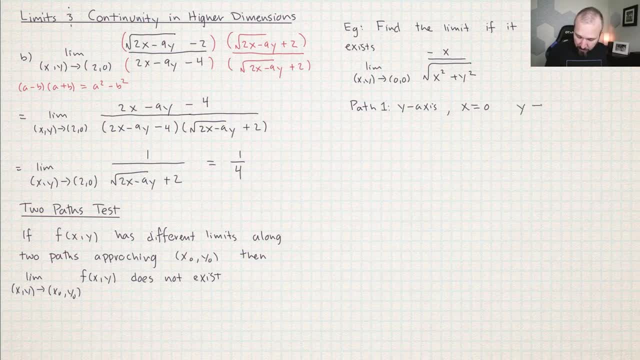 I'm going to have: X is equal to zero, And then I will have Y approach zero from, let's say, the right side. It doesn't matter, but you know I have a lot of freedom to choose any paths that I I want. Then this limit is now. it's no longer a two-dimensional limit Now, since x is equal to 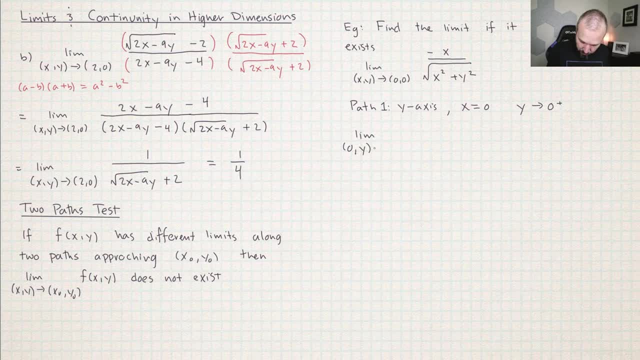 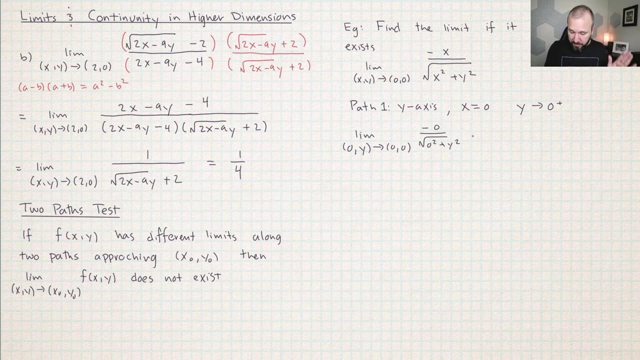 zero. this is the limit as zero. y approaches zero, zero. So on this path, x is always zero, So this is negative zero over the square root of zero squared plus y squared, So this is zero divided by some positive amount. So that's zero. So along that path I get zero. So if I choose a different, 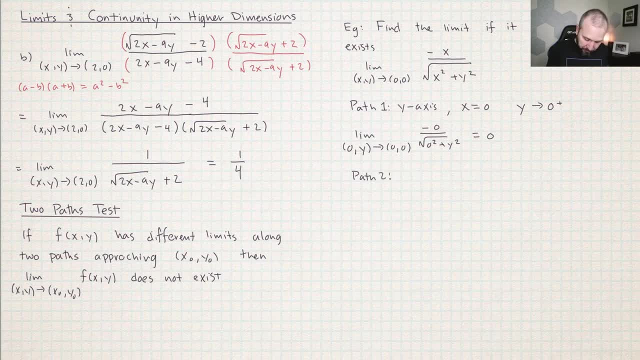 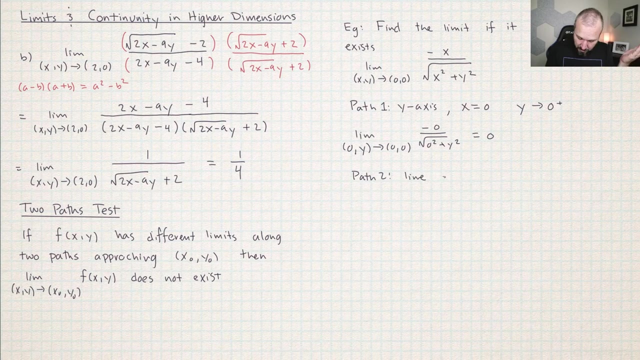 path and I get a different value for the limit, then we're done. According to the two paths test. the limit doesn't exist. So this time you have a lot of freedom to choose. This time I'm just going to choose. the line y is equal to x And in this problem I'm going to have the x's be bigger. 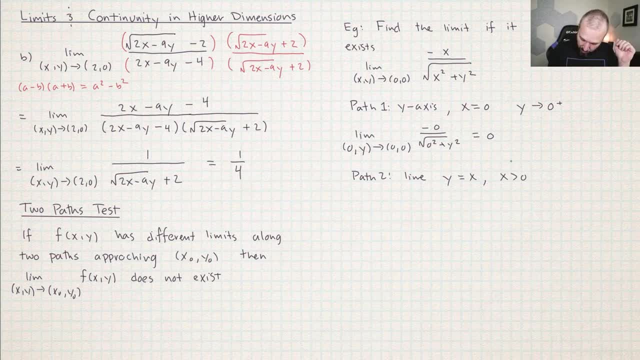 than zero. Um, so now, since y is equal to x, this is now the limit. as x, y is equal to x. So this is x. x approaches zero, zero, And these are all from the right. All of these x's are positive quantities. 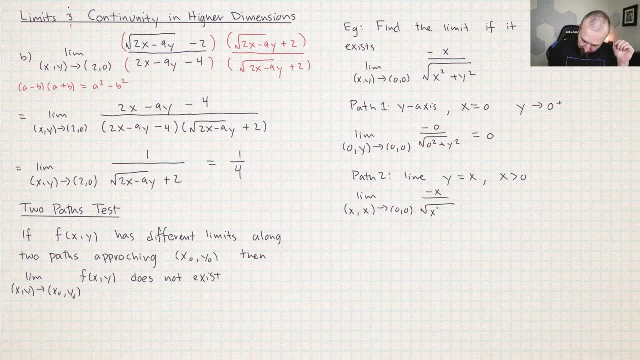 of negative x over the square root of x squared plus. Now it was y squared. but since I'm approaching along this one specific path, y equals x. this is going to be another x squared there, So I'm going to choose the line y is equal to x. So now, since y is equal to x, this is now the. 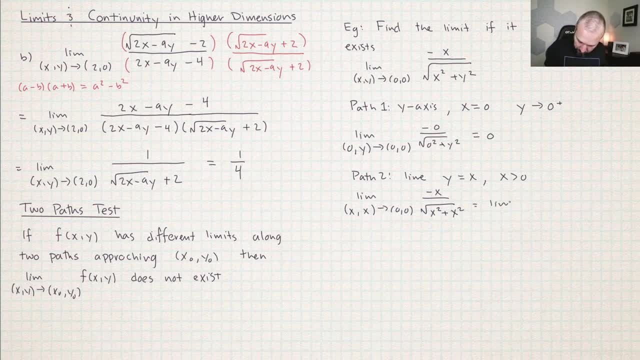 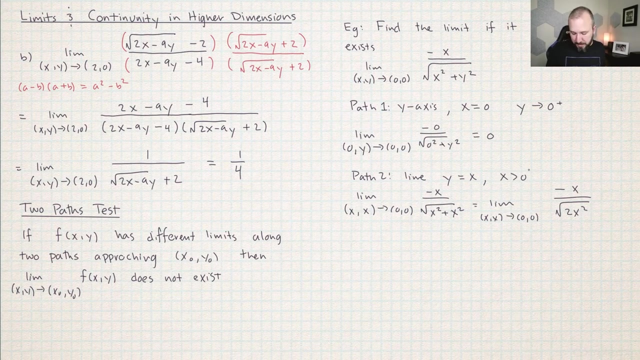 So now this is neg uh, the limit, uh, as x. x approaches zero, zero uh. but now it's going to be negative x over the square root of two x squared. So at this point, since x is bigger than zero, the square root of x squared will just be x. So I can cancel these out and I get. 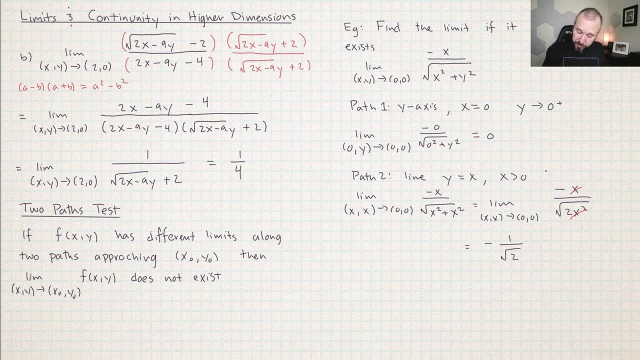 negative one over the square root of two. If I would have chosen a different path, like, say, for example, x is less than zero, then, um, I would have gotten, when I, when I reduced that square root of x, squared, I would have gotten a negative x. uh, because x would have been. 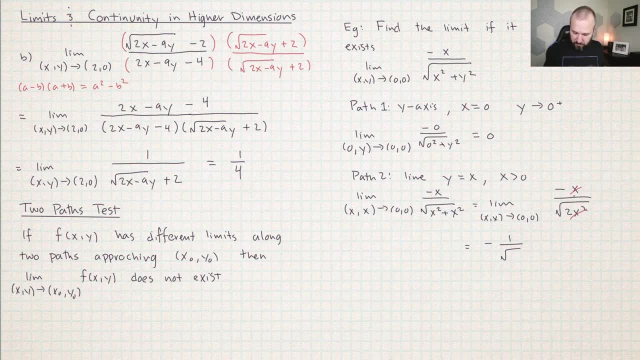 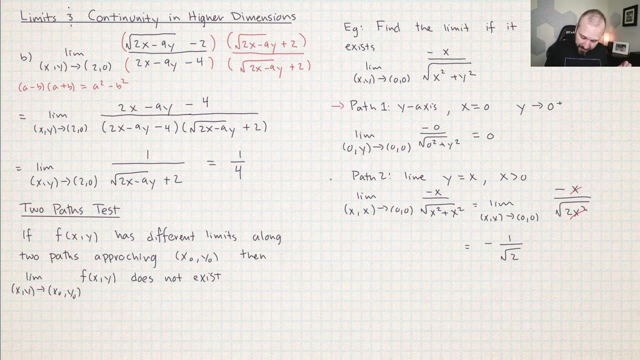 negative. So negative negative x would have been positive. again, kind of stumbled over that. Um, there is yet another way to present this, but but right now, according to this solution, we're done, because what we did was: um, I found two paths and I 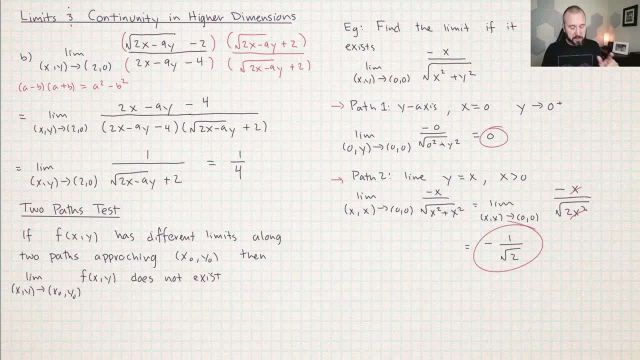 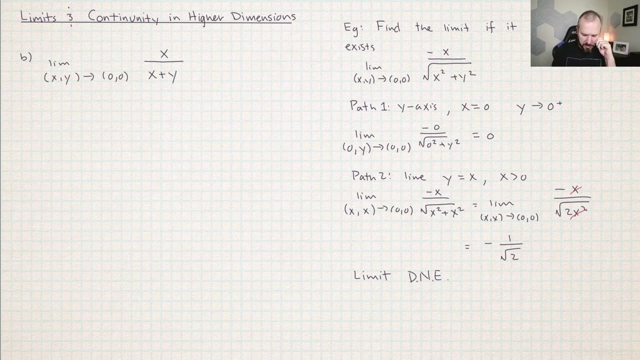 I calculated these limits along two different paths And one time I got zero And one time I got the- uh- negative one over the square root of two. So this limit limit does not exist by the two paths test. There's another way, uh, to present the solution to these two path tests. 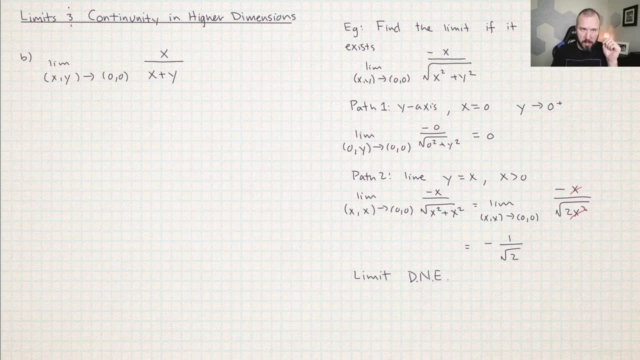 problems. I'm going to do this example of x over x plus y. Um, sometimes people just like to choose the path, So this is basically, uh, I'm going to do this example of x over x plus y. Um, sometimes, 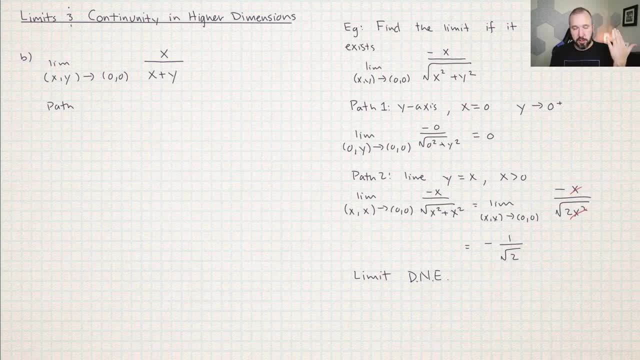 people just like to choose the path. So this example of x over x plus y, Um, sometimes like y is equal to x, but maybe I could do: y is equal to two x or y is equal to three x. So what they'll choose is they'll just do: y is equal to k times x. Um, and now along this path.